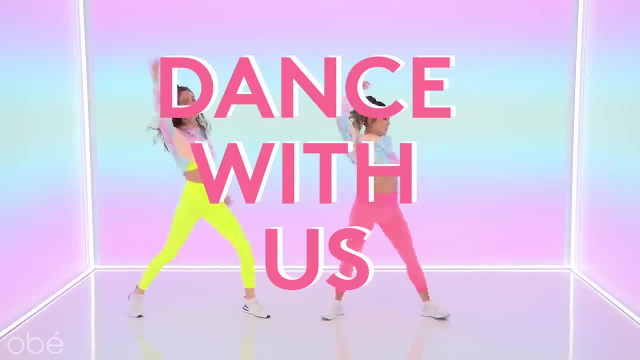 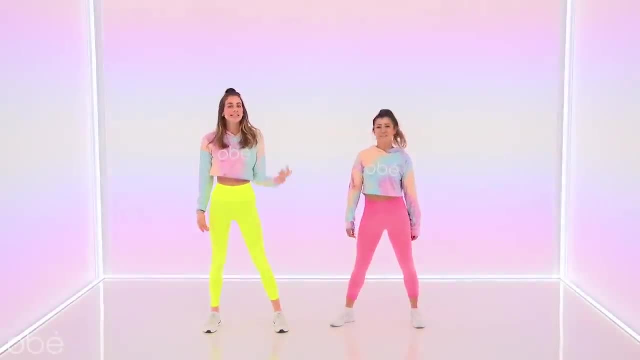 Hey, YouTube. welcome back to my YouTube channel. It's Lucy Fink. Give this video a thumbs up if you're excited to watch us dance, and also comment below and let me know what else you want to see on this channel. I'm here with Sarah Burke from Obey Fitness and she's going to teach me and you. 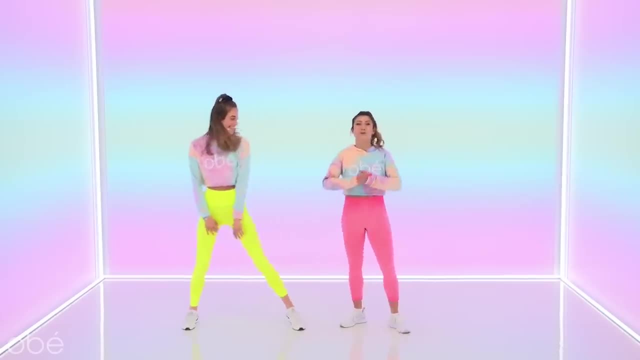 a dance right now, right here. Yes, that's right, you guys. So I'm going to break down the choreography eight by eight, step by step, and if at any point you feel like you're moving just a little too fast, no worries, Just rewind the video until you feel comfortable. Feel free to use us. 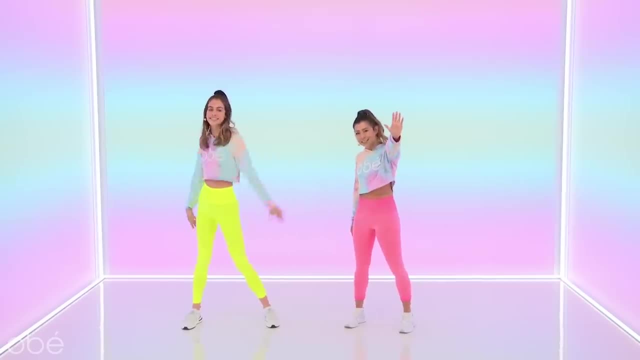 as your mirror. Yeah, so if I say right hand, it's going to be your right hand and left is their left, which is all right. So, yeah, the beauty of YouTube here is that you can just stop this video, rewind, re-watch it 150,000 times. Honestly, I'd be grateful for all those views, so just do whatever. 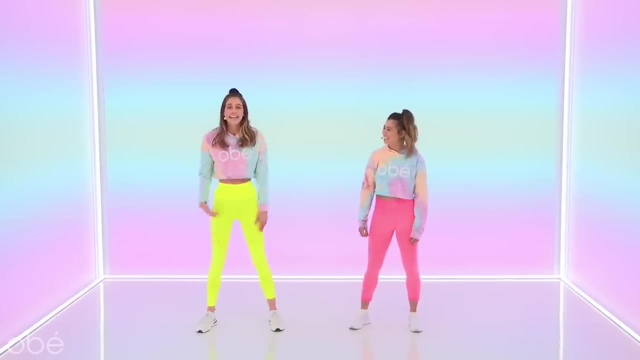 it is you want, Have fun and, just you know, learn to dance. This is my first time doing this dance as well. I have no idea what to expect and I'm not a dancer, so good luck to me and you. As I say, when in doubt, twerk it out. 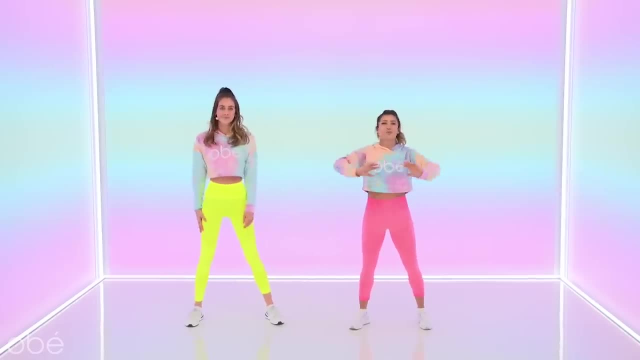 Let's do this. Oh, she did it. So if we can cut the music, we're just going to break it down for you. So I'm going to show it first and then I'll break it down. So you're going to give me one. 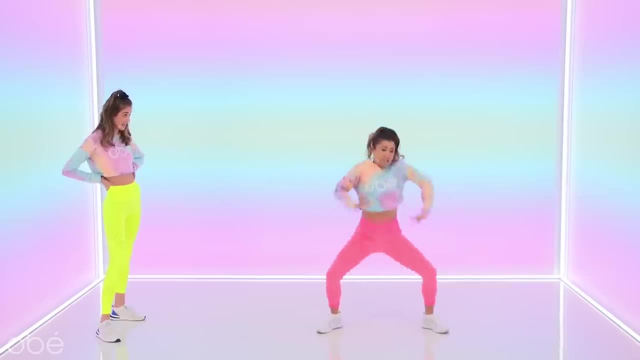 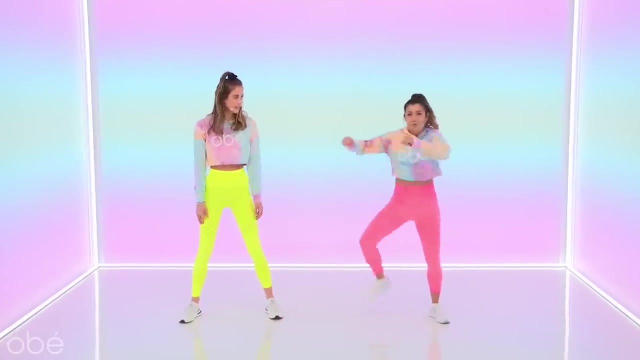 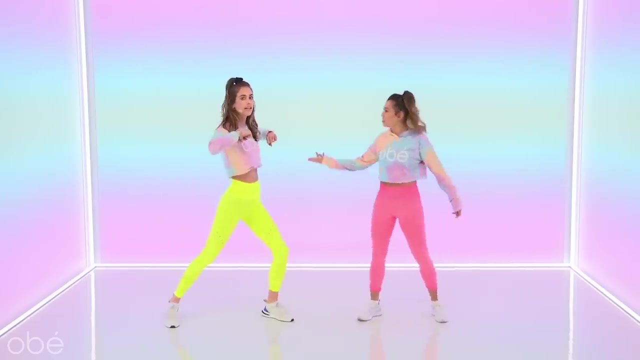 two, three and four and a five and a six and a seven and an eight. Your turn? I'm doing that. Yes, Okay, So you're going to step out with your left foot first One, And then with your right Two, First two steps Done, Hey, oh, that's it, You won. 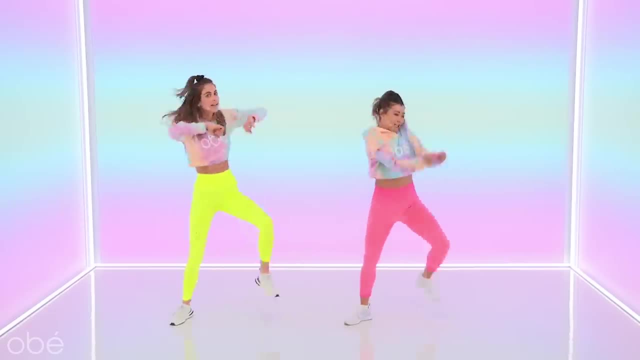 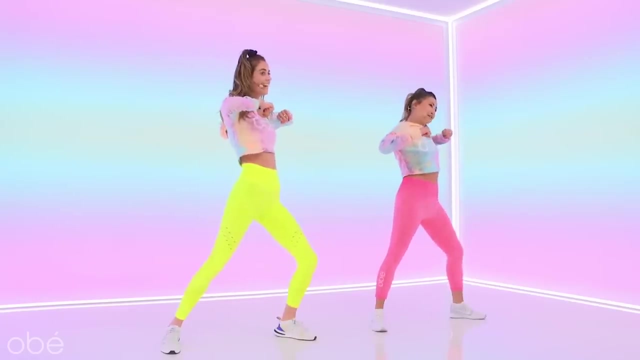 Five, six, seven- left foot goes, One, two. Easy, Just like that. Oh pro, Let's do it again. Five, six, seven- left foot goes and one, two. That's it Now. from here you're going to jump. 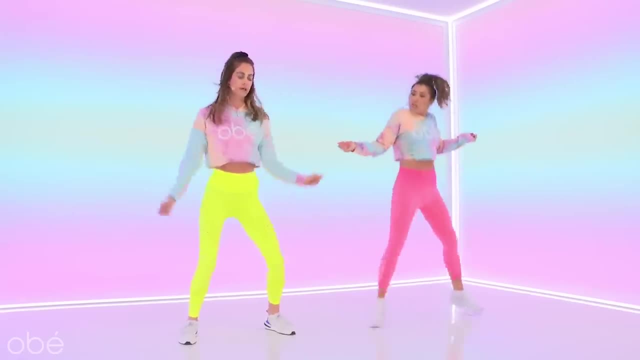 Three and just a cute crisscross. Oh nice, Three and Three and Hey, that's it. So you're going to give me three and and then on four, you're going to clap, Because who doesn't love a clap in the middle of the dance? 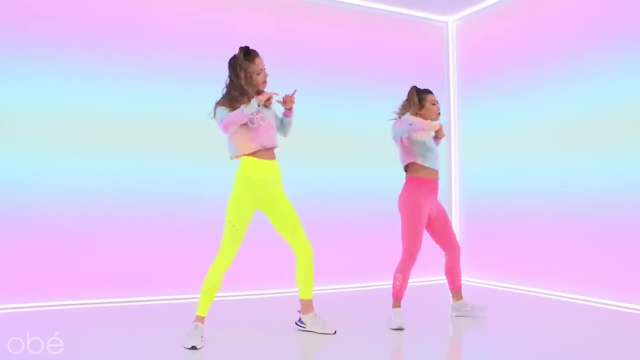 middle of the choreo. nobody doesn't love it. one, two, you're gonna give me a cute crisscross. three and four, and that's right. it is an and you're welcome and you know what I'm? I'm noticing because I'm a little taller than you. I have to. 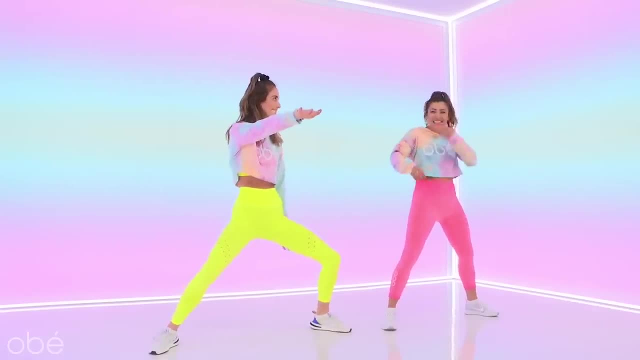 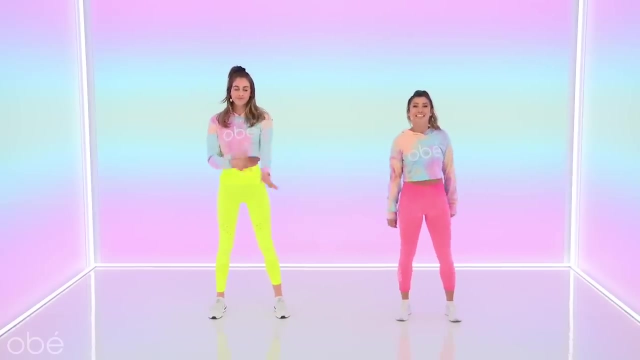 really get my legs wide and spread down here to get on your level. yeah, try to get on my level. level up, nice and slow. five, six- left foot goes and one, two cross, three and four. did you do it? I think so. did you. five, six, seven, eight? 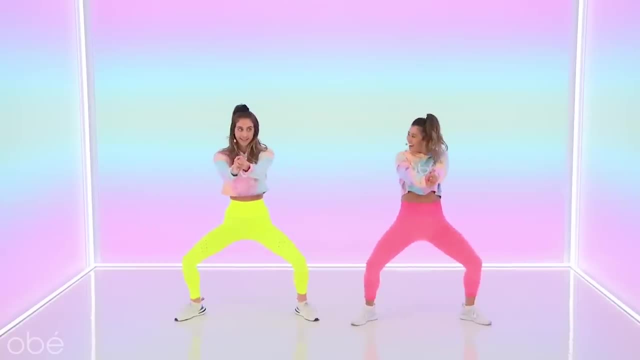 and one, two cross it. three and four: hey, oh, it's just slightly faster. oh, how much faster. okay, five, six, seven, eight and one, two, three and oh yeah, that was such a solid clap from here. after you clap, you're gonna bring in that left knee. five, hey, oh, bring in that right. 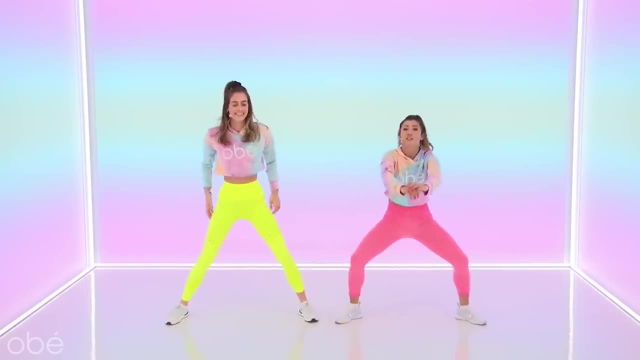 oh, that's right, so you're gonna pull it in. pull it in so it's gonna go five, six and you're gonna give me a roll seven and then drop it lower, eight. when we did this knee thing, are we pulling our arms in with it like yes, please, yes, please. 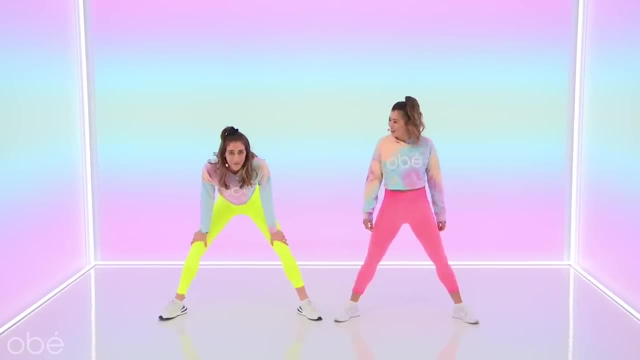 okay, you know my thighs are a little sore, just know it's my, but actually you know, tone up, yeah, so let's take it again from that in and then roll it on down. great, yeah, one, two, three, four left five, six thin chest, roll it down. oh, did you do? 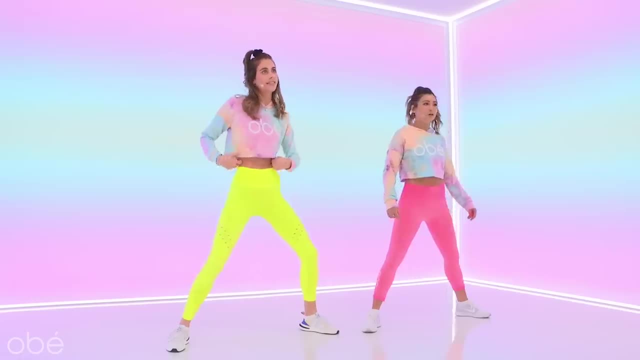 it. I think I did it, but you know what? I don't. my whole ribcage isolation thing doesn't come as naturally as yours. you're doing it. you just want to make that obey move around the world. oh, oh, I like this direction. hey, from the top. 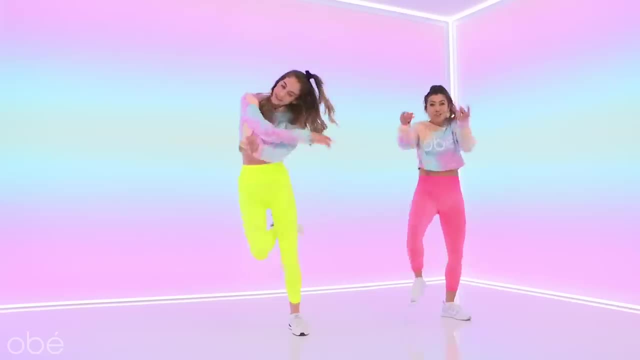 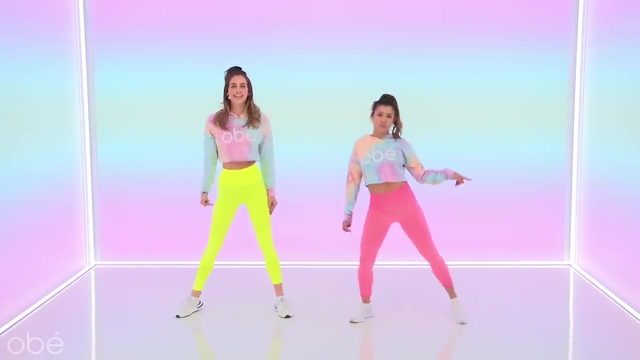 yeah, five, six, seven. left foot goes one, two, cross it three and clap it. give me left, give me right, then roll it on down. nice, eight, done first, eight, done, eight, done first eight. and how many eight do we have? four, four, eight counts. we are 25% done with this dance. five, six, seven. 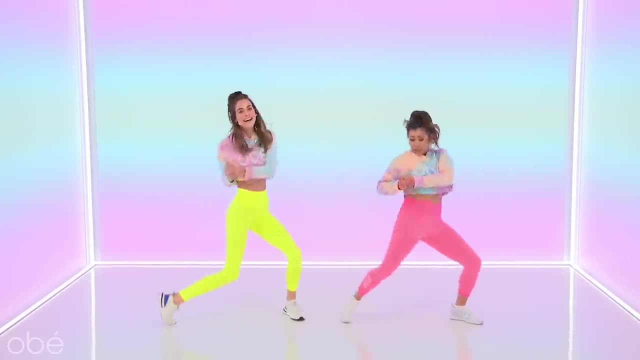 eight and one, two, cross it three and clap, give me left, give me right, then roll it on down. wait, by the way, everyone, Sarah choreographed this entire dance herself and we have this incredible jingle punks track to play it, to which, if you don't know, jingle punks is it's license-free, copyright-free, royalty-free. 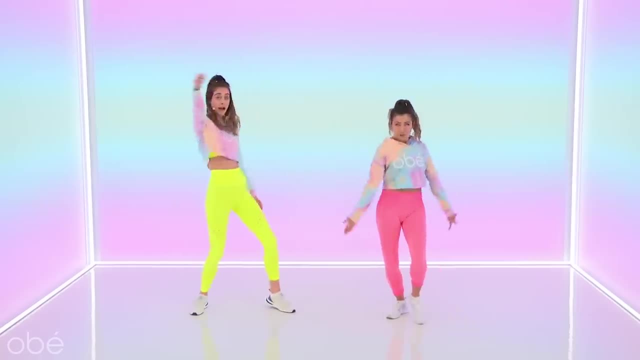 music that we are gonna play for you right now. yeah, let's go killed it and I could get the music. gods, tell me when we're starting. I'll always count you in. okay, ready, five, six, seven left. give me, let's give me right. yeah, five, six, seven, eight. 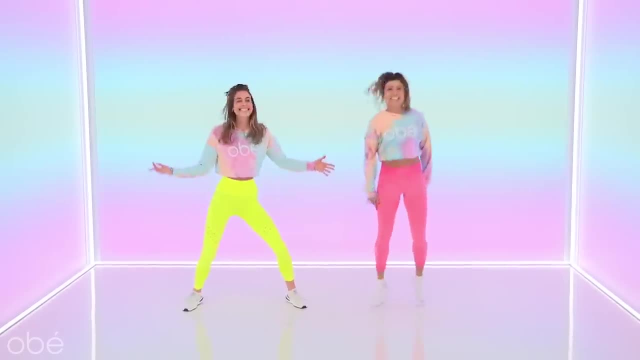 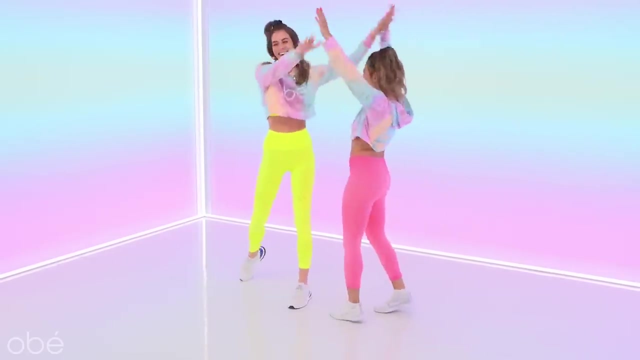 I wasn't breathing. gotta get the oxygen to the brain. hey, I got that flow. there's five, six, seven. here you go, three and four. bring it in. bring it in, then roll it on down. I was breathing that time. I was breathing that time. okay, thank you, music gods, and, as we said, if we're moving a little too fast, 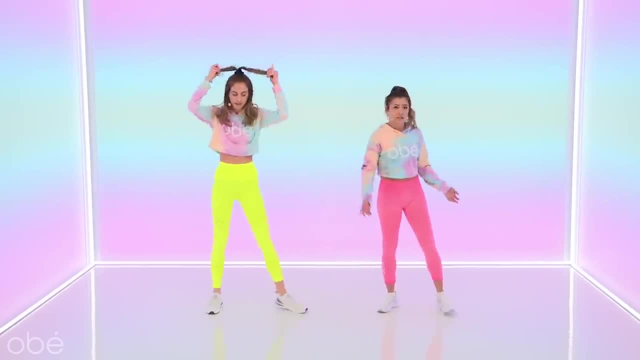 just rewind it. pause, rewind YouTube. but you're getting so fast, like so you have seven, eight. I'm gonna show you the next thing: okay, okay, ready. so you have one, two, three and four. you drive it. five, six and a seven, eight. oh, you gotta pull a. 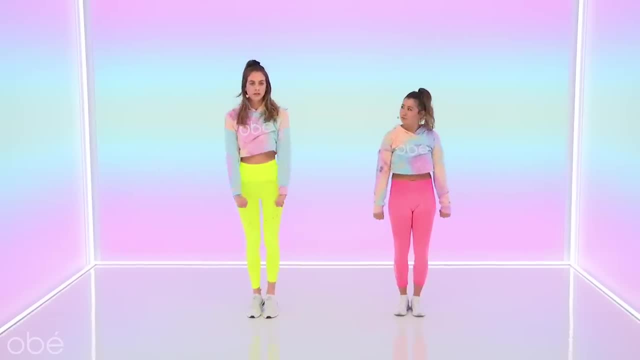 blanket over your chest. one, one, two, yeah, that's it, which is gonna feel great, cuz you just went lower, lower. yeah, it's like after you get down and your legs are just about squatting. you get to stand up straight from here. you're gonna step out with your left. 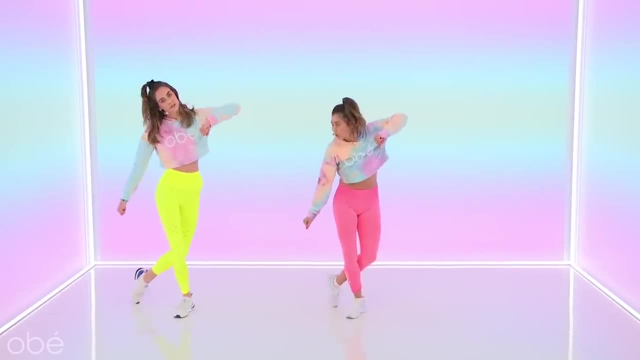 three and four, you tuck that right. Oh, perfection, that's it. that's kind of like it's cheerleader move, hey. so in case you're like: who, what, what, what you're doing is you're just pumping twice, so you're going left and then down. so 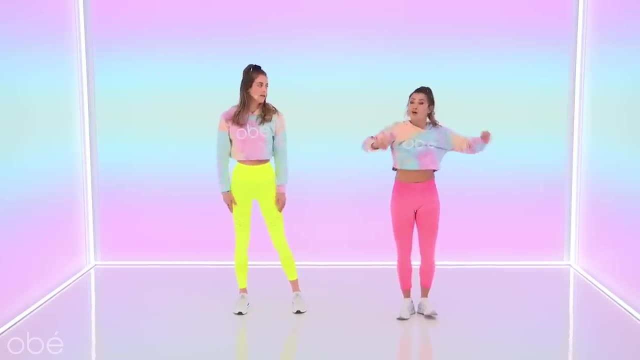 you're hitting that upper corner and then lower corner, you're gonna give me three, four, so let's try that. so just to confirm this: this right elbow, is it going diagonal up and then diagonal down, please? yeah, i would love that. so you just did one, two. 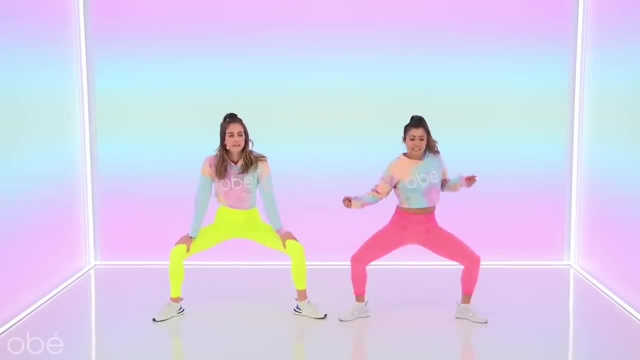 step out left three and four, five, six, seven, up and over one. two step left three, four. it's just slightly faster, though. okay, can we do it from this clap? yeah, you want to. yeah, so this is four, and then you do the five and the six, just in case you're like: oh my god, where are we right? one, two. 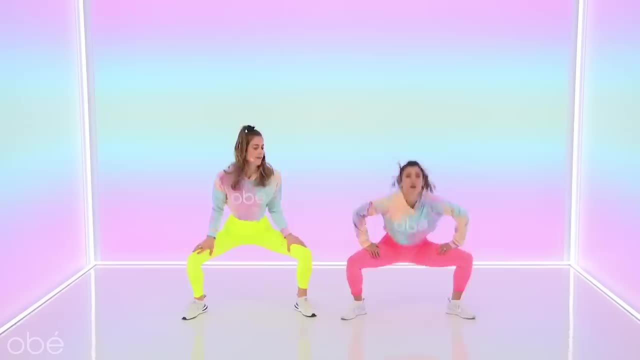 three, four, bring it in, bring it in and bring it on lower. and one, two and a three and a four. we should just finish this. eight, okay, okay, yeah, three and a four. you're gonna drive it over five, six, so you're gonna go right left, hey, and then you're just gonna stick it back out. seven cross our eight. 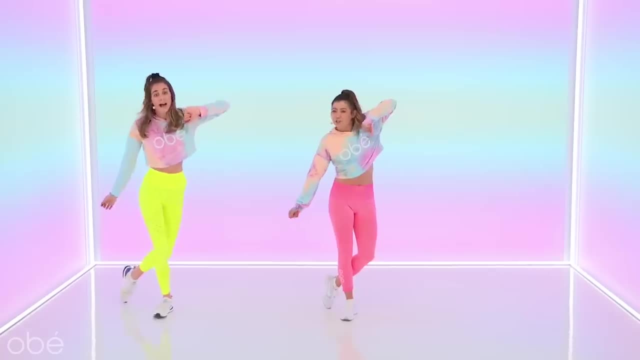 lost my balance there. we're driving a car. we're actually taking our left hand and going drive. yes, car, it might be a spaceship. back it up, move it forward. yes, okay, you know, because it's a really big. if anyone out there has their driver's license, you should know. 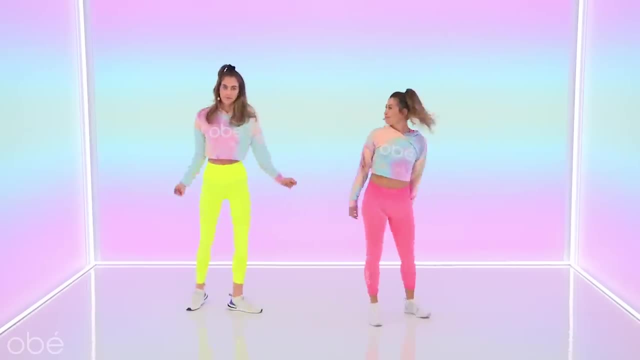 this move, hey, from the car. hmm, great, that's the whole eight. that's the whole eight. yeah, oh my gosh, we are cruising. we're actually in a car from this. you have one, two and you take it over three and four. you drive it five, six, stick it out seven, cross it eight. oh, let's connect everything just. 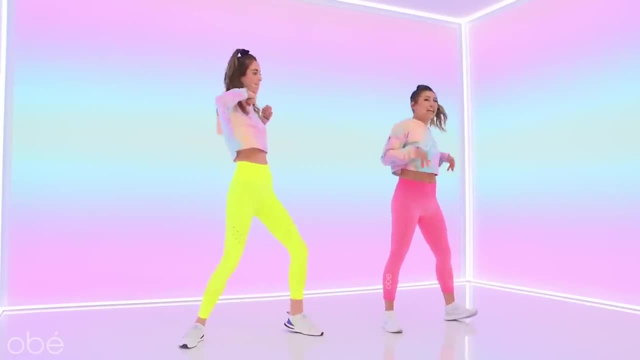 in case we forgot how it started. it goes like this and then it goes like that: that whole thing great. five, six, seven, eight. step it one, two, cross it three, clap it four, bring it in. bring it in then higher, then lower up and over two, three and drive it five in the car and seven and four. that's it, five, six, seven left. 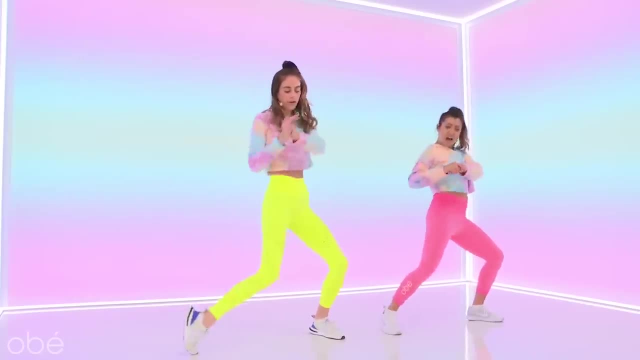 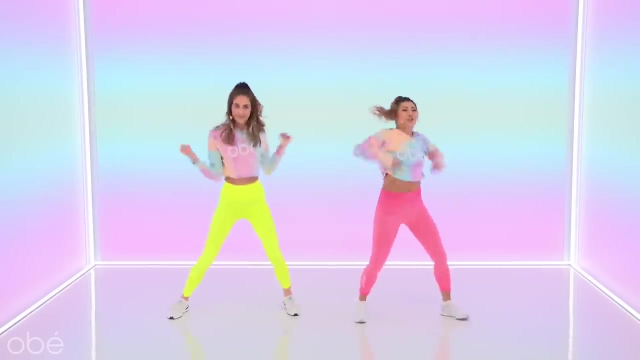 one, two, three and left knee five, six, then a higher than a lower up and over left three and four. driver five, six and seven, eight, except it's faster: one, two, five, six, seven, eight and one, two, a three and four. bring it in. bring it in, then bring it on low. one, two and a, three and a four. drive it. five, six and a. 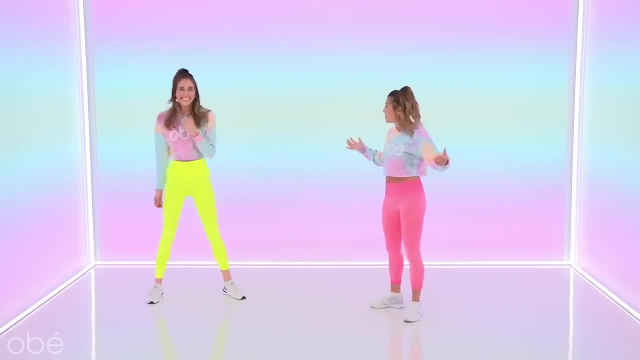 seven. i'm having so much fun. yeah, yeah, i'm so glad. i hope you guys are having fun too at home. yeah, if you're having fun, comment below and let us know. listen. you should just dance like no one's watching. oh wait, are you at home watching youtube? no one is watching. go crazy, and you know what if? 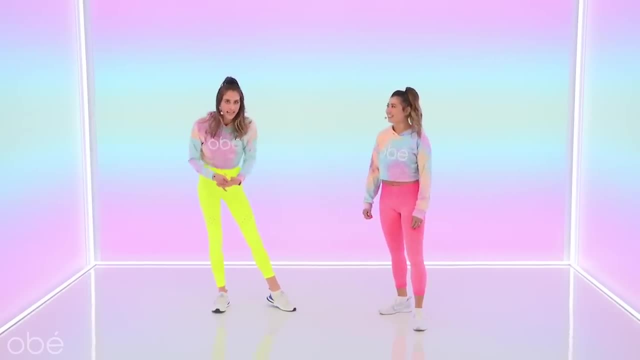 you do want someone to watch record yourself, put it on social media, tag us. oh my god, we would love. we will repost it always on my honor, all day. let's try this music. music guys. they knew i love this song. five, six and bring it down up and over to the left drive. 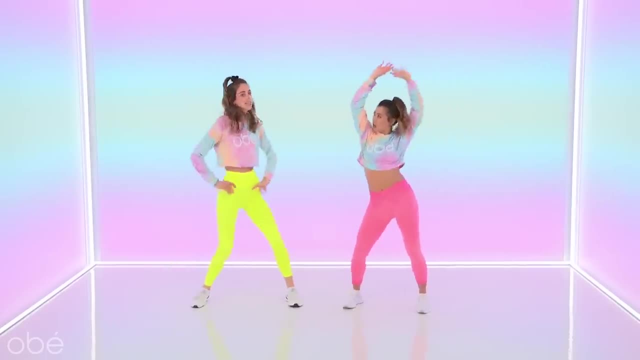 Hey, this is like my favorite dance that ever done, ever, ever, Oh, my god, Thank you. Five, six, seven. You breathing, I am, You know, I kind of like the idea of breathing with the moves. Hey, oh, you're giving me vowels, Ladies and gentlemen, pro, So after you cross it. 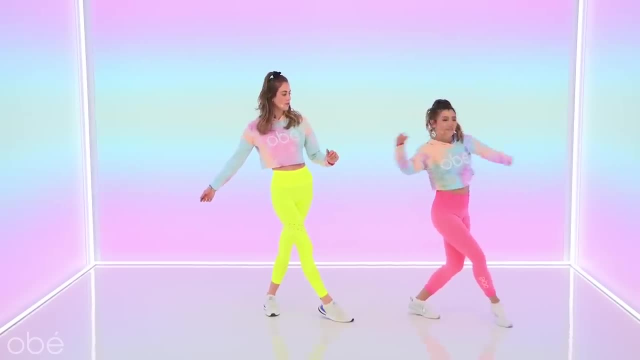 Eight, I'm gonna show you. you ready. You have one, two, uh three, uh four. you slide it five, pick it up six, drop seven, eight. Oh, I've always wanted to know how to do this. So your left foot is crossed. now you're prepped for a turn, So you're just gonna pivot to the back wall. 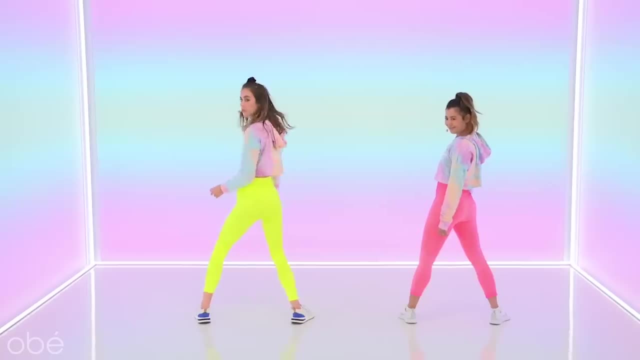 Now you can't see us, but we'll keep talking to you. Mm-hmm, We're still here. We're still here. Now It's gonna be your right hand, You're gonna put something in your back pocket, Put it in. 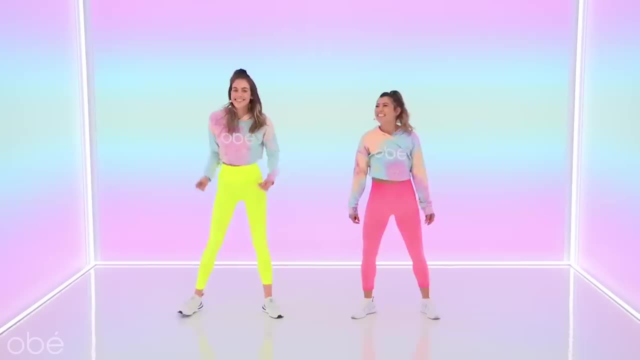 Now put something with your left in the back pocket, Go, go. So after you cross Seven, eight, you bring it around. one, two, that left hand is gonna go back, and three, now your right. and four: Just put them in your back pocket and save it for that rainy day in the pocket. 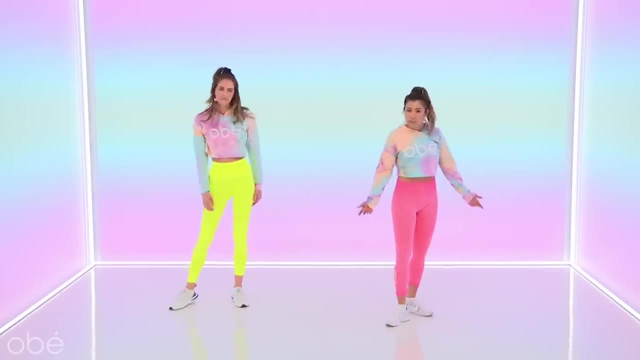 If you do the wrong arm, who cares? No one's gonna see, no one's gonna judge, We're never gonna tell I don't care. So you have one, two and a three and a four. you're gonna slide that left leg in on Five, pick her up on six. Whoa Hey, drop her down seven. 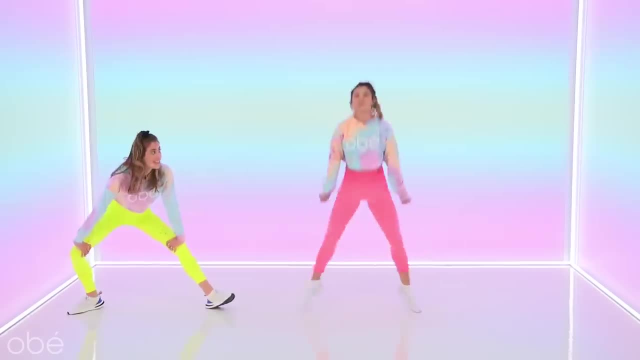 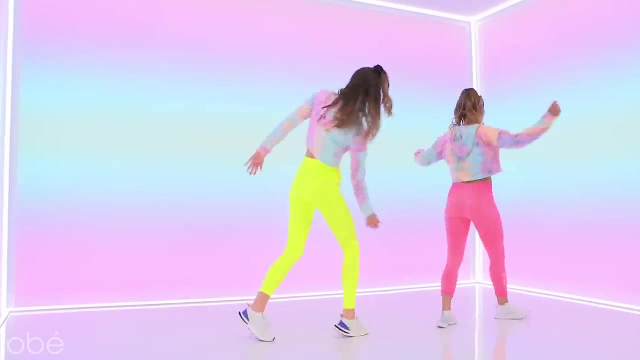 This is not good for the thighs. They're lucky for you. We just push them off and jump together again eight. So to recap that move: we drove Mm-hmm the car and then you bring it back in, that. you bring her around one to back pocket a three. 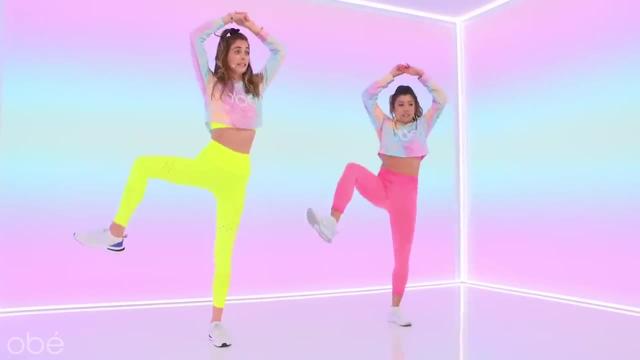 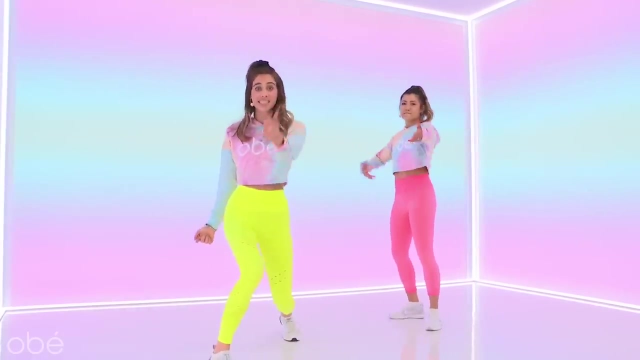 For slide that left and five pick her up, six to drop it down, seven then bring it up. I tell you, yeah, you're seven, eight, 25% done. You're almost at the stage where you can perform this dance and feel like Sarah. 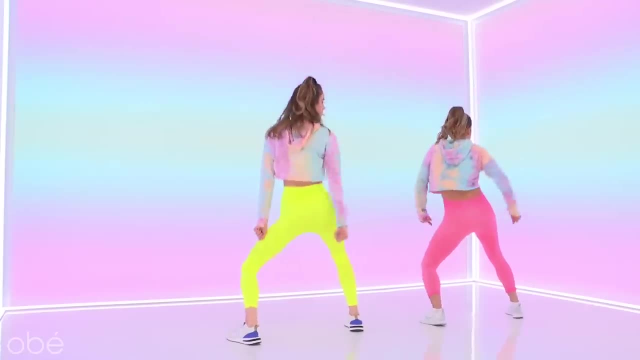 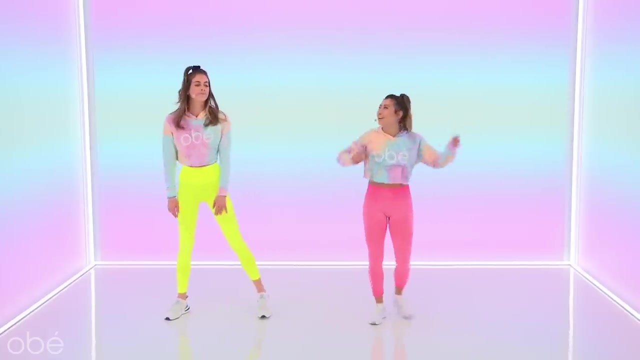 Pivot one, two, put it back a three, a four, slide it five, bring it up six, drop it seven up eight. Should we take it from that? Blink it one, two, then a three and a four, five, six, seven, eight, up and over one. 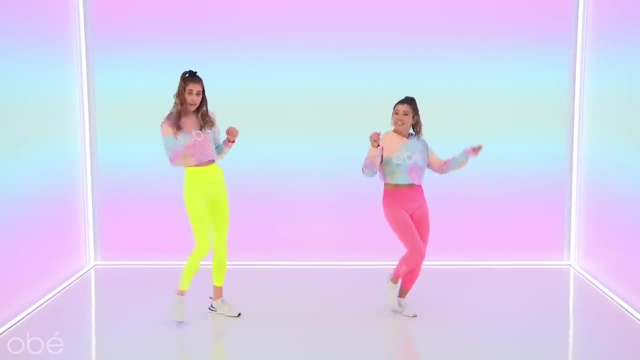 two to the left, drive it five, six, then seven, cross it pivot one, two and a three and a four, slide it five, six, drop it seven, eight, five, six, drop it seven, eight and. 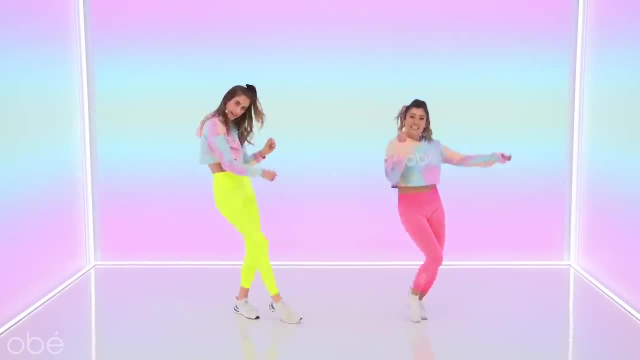 one, two, three, four, drive it five, six and seven. cross it eight and pivot yes, a three, four, five, six, drop it seven, eight. Before we move on, I need a sip of water. 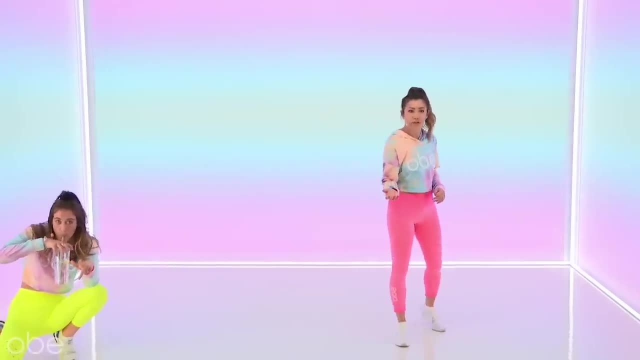 Oh, get a sip of water, Take a water break. You're more than welcome to have some water. Five, six, seven. left foot goes one, two a three and clap. give me left, give me right. 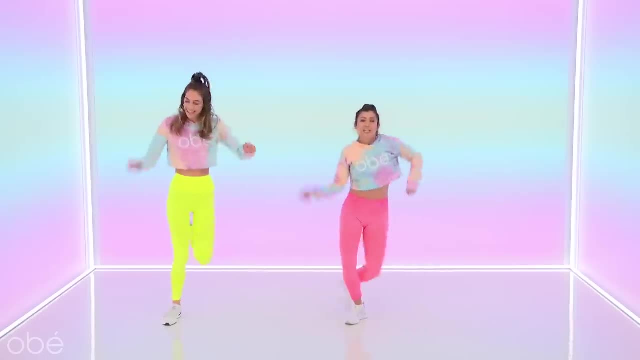 then roll it on down And one, two, three, four, five, six, seven, eight and a four, slide it. five, six, drop seven. one, two to the left, drive it and seven. let's pivot one, two. 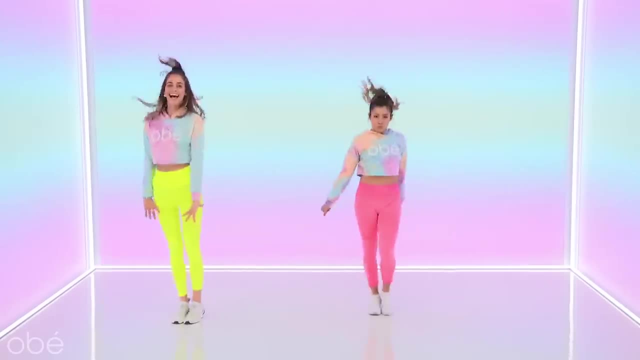 three, four and five up six, drop seven one more time and then we'll bring in the music. Five, six, seven, eight left one, two, three and four, five, six. then roll it on. 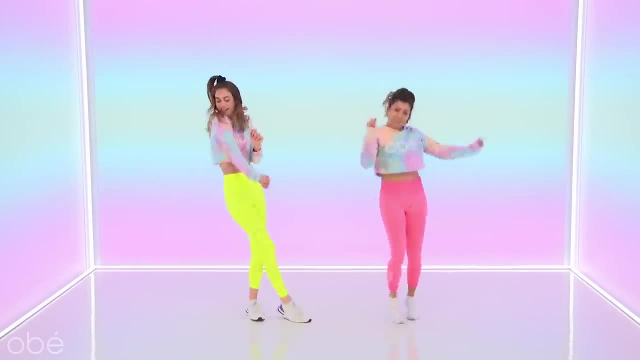 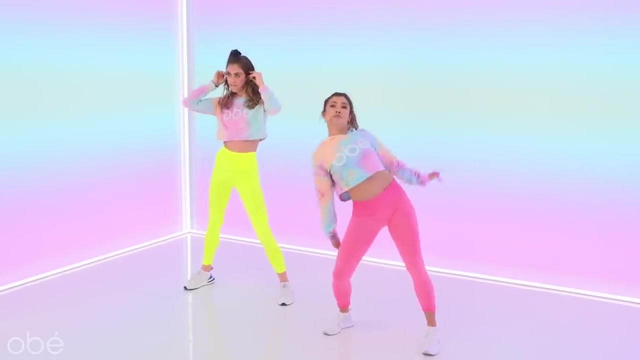 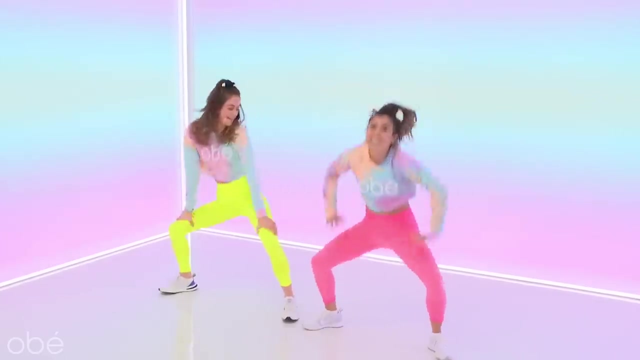 down and one, two, a three and four, five, six and a seven. let's pivot one, two, three, four and a five and drop it up. ั่� Lloya, Hey, hey, up and over. three and four, five, six, seven. pivot one, two, hup, hup, go. and five, six, hey, you ready? yep, five, six, seven, hey, hey, and bring it on down. and one, two to the left, seven, pivot, one, two, hup. 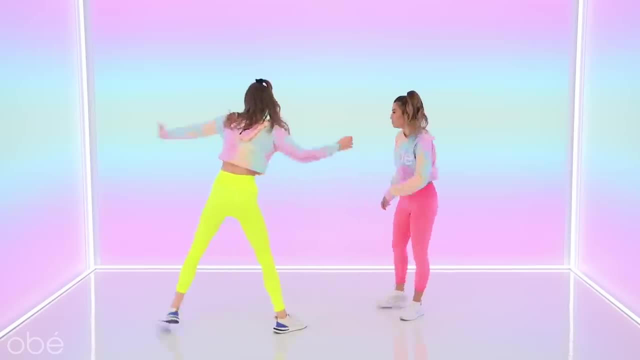 three, hup four and up. I go down, perk, bend and snap. this is the last eight. I don't even know how we, how we got this far because of you, but here we are. if you come in with a good attitude and you're ready to go and you just went in doubt- twerk it out. you're gonna learn the whole thing. just have fun, because this is youtubecom. so you just snap back up. you just said bend and snap and you're gonna give me one, two, three, four- you're done- five, six. then twerk it on out. 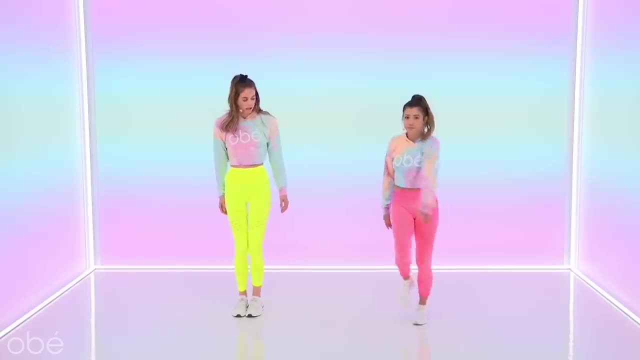 so we snap, snap together on eight. I'm gonna step out with your left step, so make sure you can see your face. try not to cover it, because you never want to cover the goods. from here you're gonna sit center, center- oh, I gotta get lower. and then from here you're gonna step right with your left arm. again same thing, don't hide the goods, press that chest out and then sit center. hey, hey, break that stage. girl, should I not be pushing as hard? I feel as if my microphone is falling off my head. so when you step, 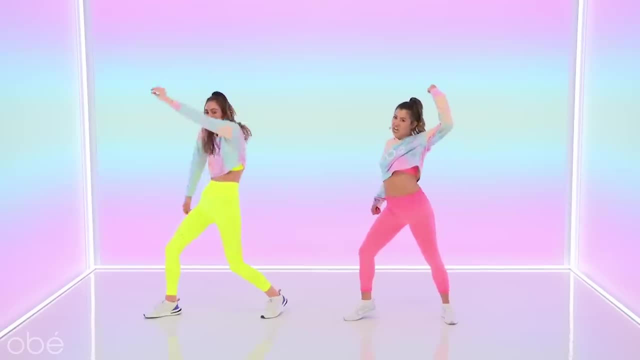 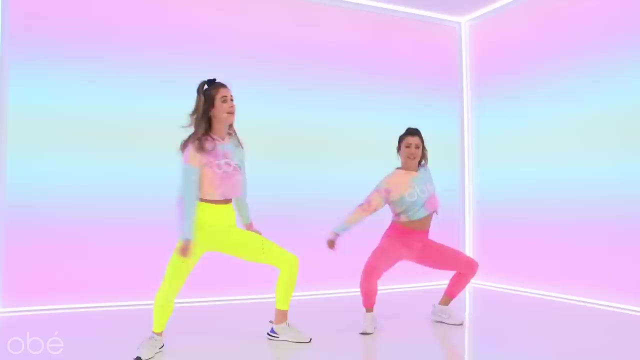 really think about pressing out, like as if you got a new like push-up bra and you're like, look at it, so proud of it, then, from here, sit center. and then you're like, also, look at the other side of it. we just snapped up left leg. five, six, seven, eight, step one to center. 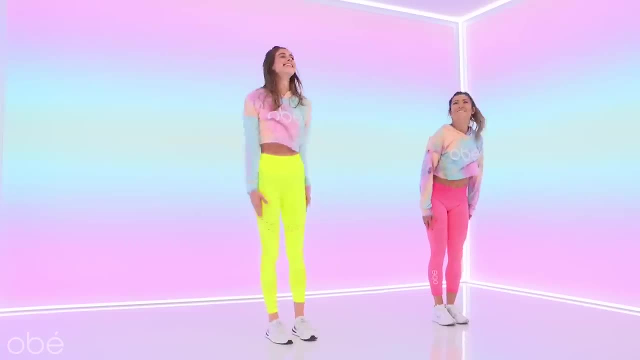 then step to center. did you do it? I did it. five six seven left, one, two, three, four. five six seven left and one, two and a three, Four. from here you're gonna give me two jumps. 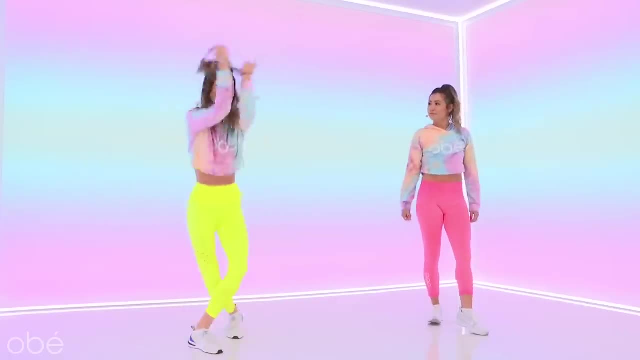 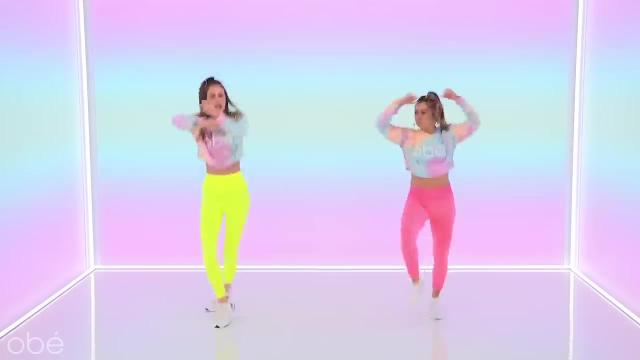 cross it out. Hey, can I say? Yeah, I didn't know it was Christmas, because you about to crack a nut, because it is Nutcracker time. Oh, What a funny dad joke you just made. You're welcome. You know, I sometimes crack nuts on other holidays as well. 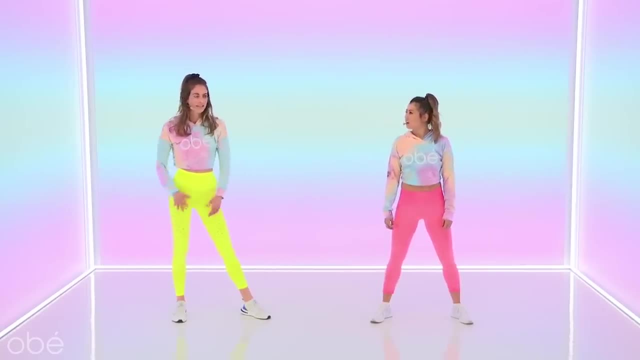 Like what kind of nuts Thanksgiving? we bring out the Nutcracker. Oh, You just went one, two, three, four Nutcracker. You're gonna jump left and then right. I love the way your jumps. you almost do like a. 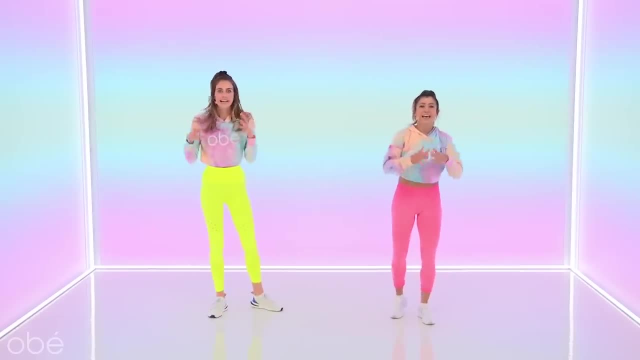 like a double jump really fast, but it's so fast that you can't even see it. It's just an extra bounce where you're just like: Yeah, you're like I'm gonna try it, but I can't guarantee it. 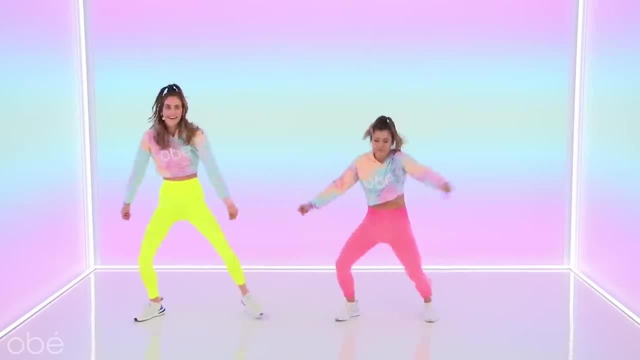 Okay, five, six, seven. left One, two, three, four, jump it, jump it. Last bit, you're gonna twerk it out. Oh, You jump back out and you give me this amazing fist pump. Seven and eight. 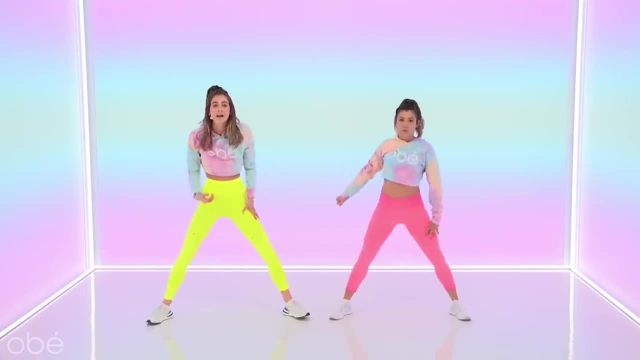 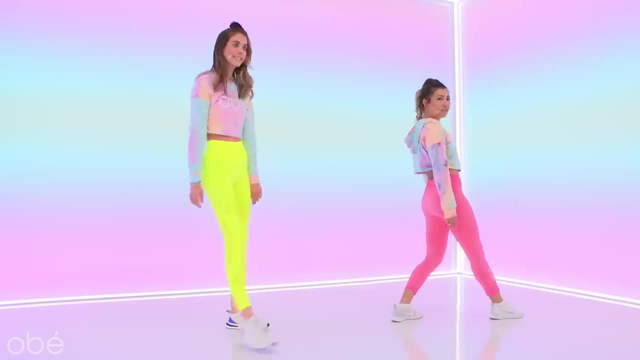 So you go. Oh, it's that fast. Of course you're welcome. We did it. Yes, that's the whole choreo. you guys, we did it, That's it. That's it. Pivot, like Ross from Friends. 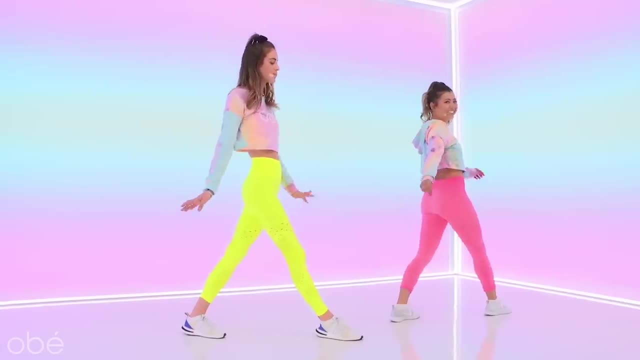 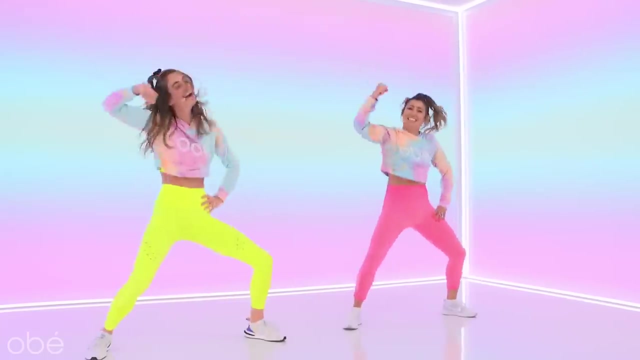 Pivot: Exactly, pivot, Yes, five, six, seven. pivot One, two and a three and a four and a five, six. drop it seven: Left one, two, right three, four. Nutcracker: five, six and. 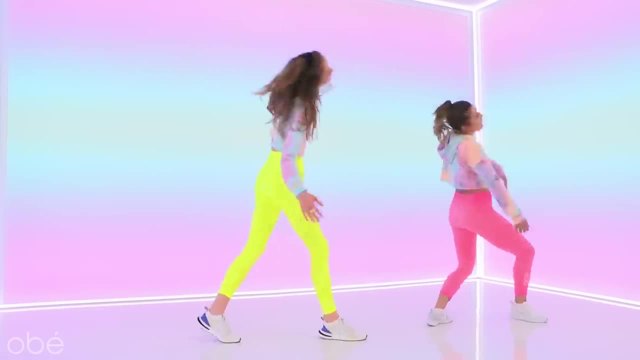 Ready, Yep, Five, six pivot and one, two and a and a. slide it five, whoop six, drop it seven And a left two. that's okay, you just keep on going to go. 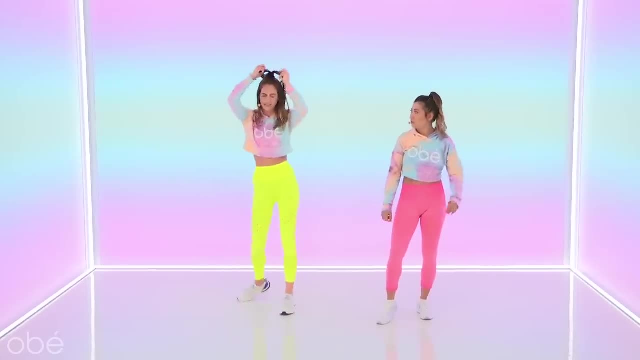 That's it. it's just that it's faster. Okay, I remember that it's faster. every time the music comes on, I forget that. I re-remember Five, six, five, six, seven. pivot one, two and a three and a four, slide it five, whoop six, drop seven left leg. 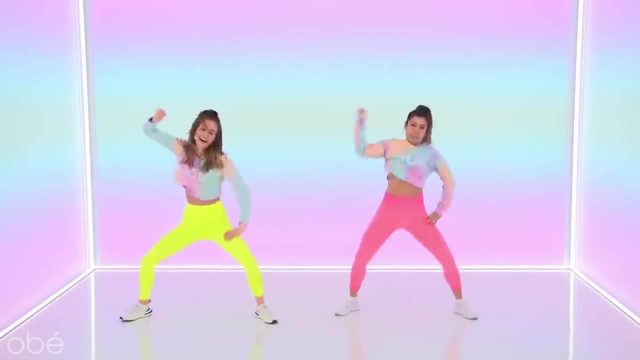 One, two, three, four, Jump it five, six, then end it with a twirl: Four, eight. counts down in the books in the box. How did you do at home? Let us know, Just to make sure we remember everything. let's take a cute little walk from the top. 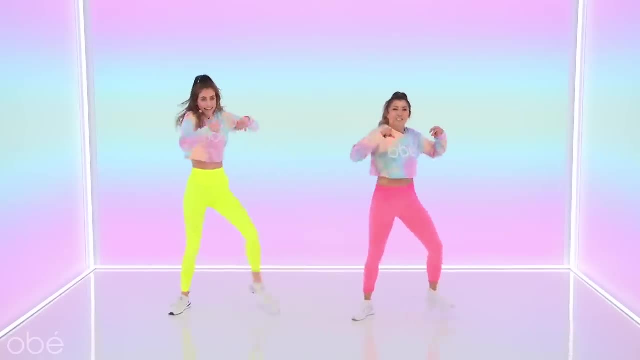 Five, six. left foot goes one, two a three and clap: Give me left, give me right, then bring her on down. and one, two to the left, Drive it five, six and seven. let's pivot. 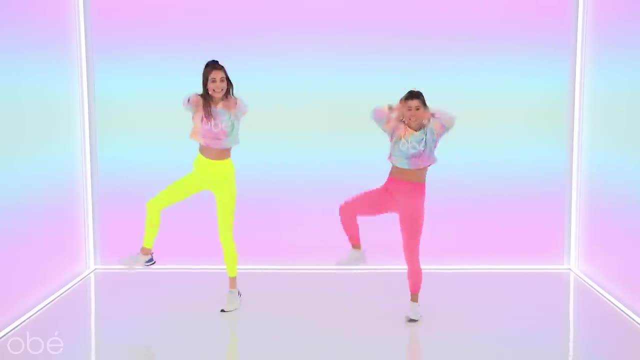 One, two and a three and a four. slide it five, whoop, six and seven. left leg: One, two, One, two and a three- let's nut crack her. five, six, then end it with a twirl. 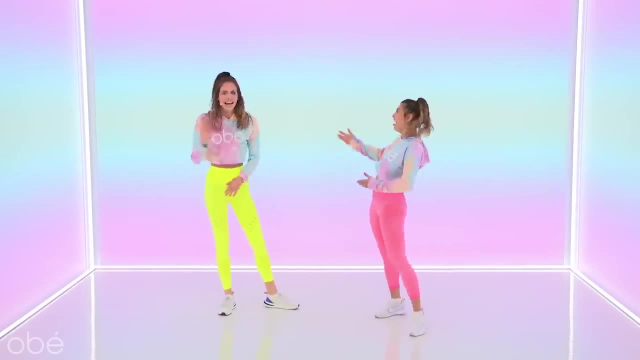 I did it all, You did it all. I didn't even mess up, Not that that matters or anything, but it does matter. Five, six left, Hey, hey, drop it low edge And drive And pivot. 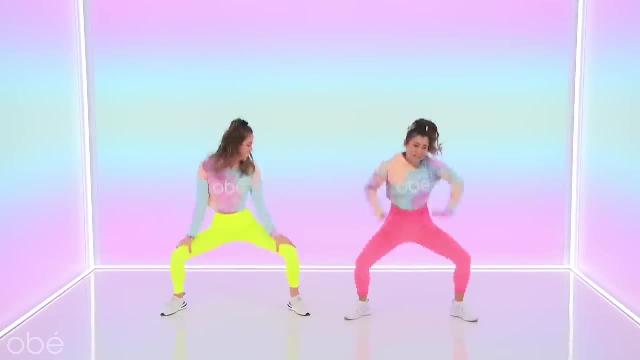 And three and four and five, six left leg goes, Let's nut crack her. And three and four and five, six left leg goes, Let's nut crack her. Five, six and a three and end it with a twirl. 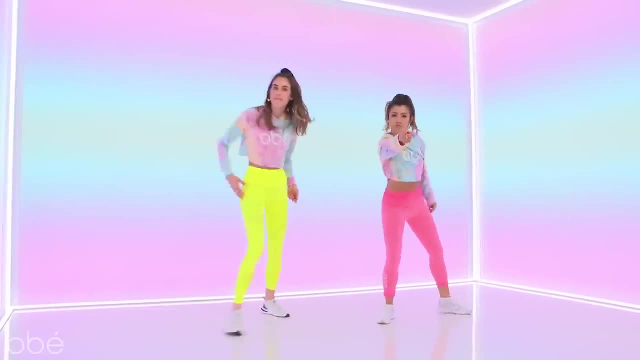 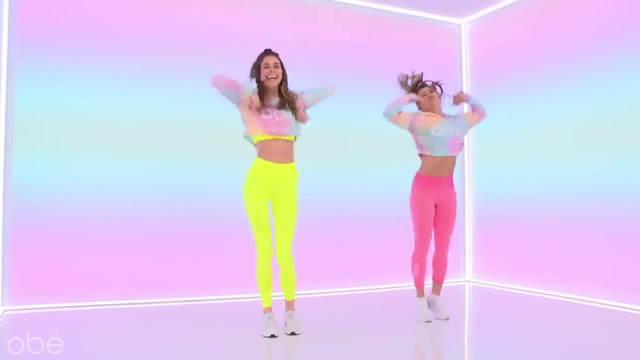 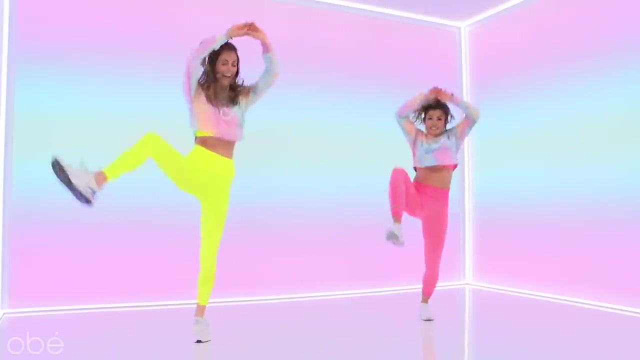 And twerk it, Woo. Should we look right in this camera and freak them out? Five, six, seven, Hey, hey, Woo, Are you guys breathing? Let's pivot. Hey, hey, Left leg Nutcracker. 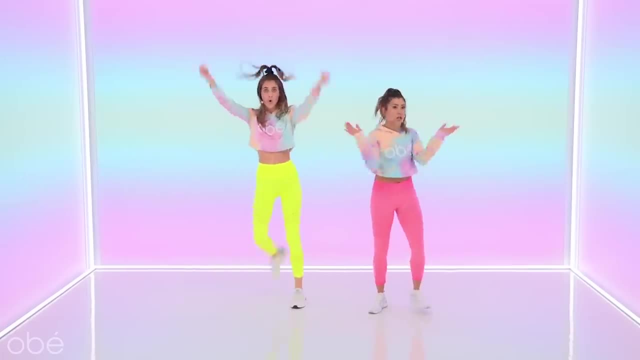 I'm dying. Five, six, seven, Up to the rib cage. Hey, I don't got time to show you how. You already know that I get down. If you wanna see me, bring the crab. I chop ish up to my first name. 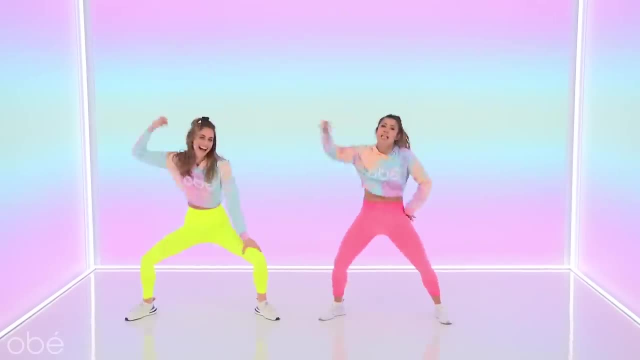 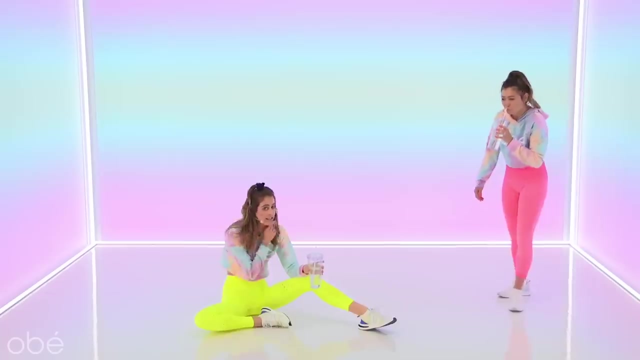 Yeah me, I'll bring heat to the one I freeze them up in twing Woo, Let's take a moment, Catch your breath, Get some water, Set up yourself. This is cardio for me. Listen, dancing, it's everything. 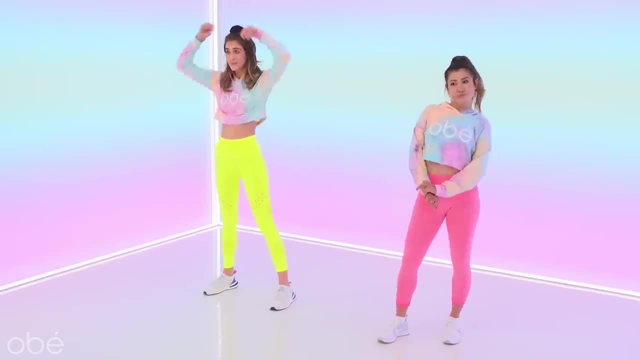 All right, last few times to marathon it, and then that's it. Kabaddi kabaddi, Don't forget about your intro too. Kabaddi kabaddi, You're allowed to move before the choreo. 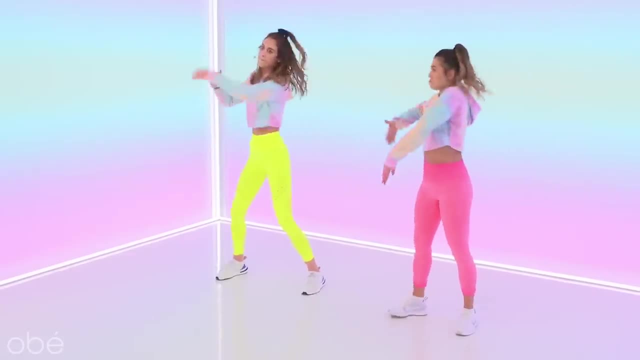 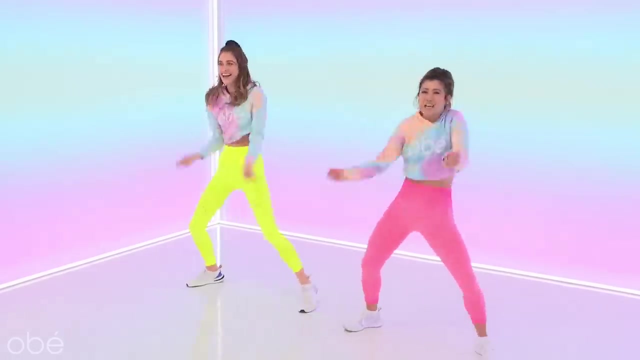 Kabaddi, kabaddi. Should we choreograph our intro? Oh, Milly rock, I got that. Hey, Five, six, seven. You're gonna feel it like a jab right to the rib cage. Hey, hey, and bring it down.